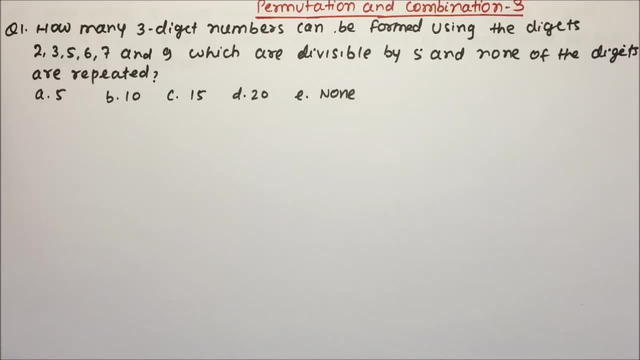 And friends, our today's, our today's question is very, very important question. I am putting little force on that because our today's question is really very important question and you need to understand how we can solve this question. So, friends, let us start with the. 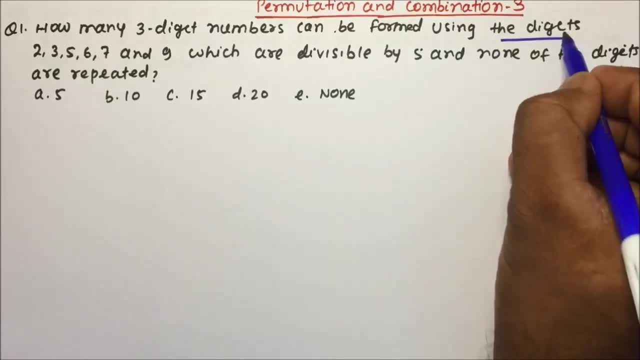 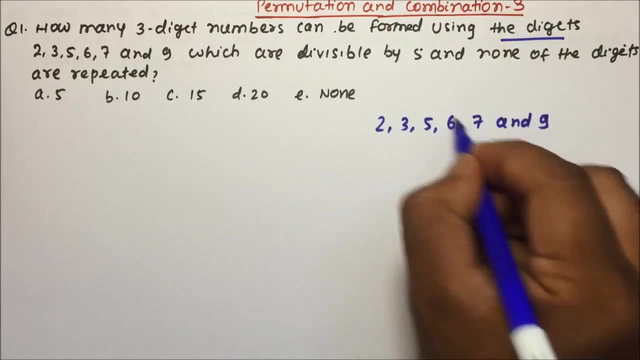 question number 1.. How many 3 digits number can be formed using the digits 2, 3, 5, 6,, 7 and 9, which is divisible by 5 and none of the digits and none of the digits repeated, And digits are. 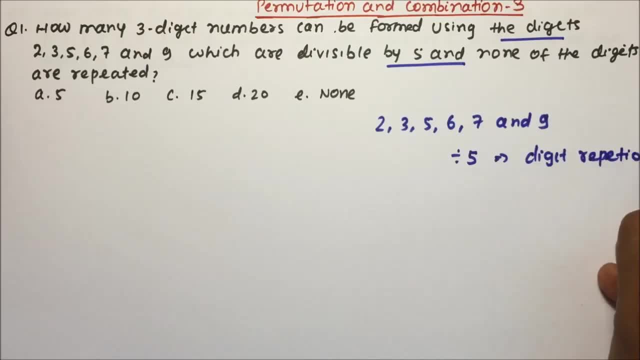 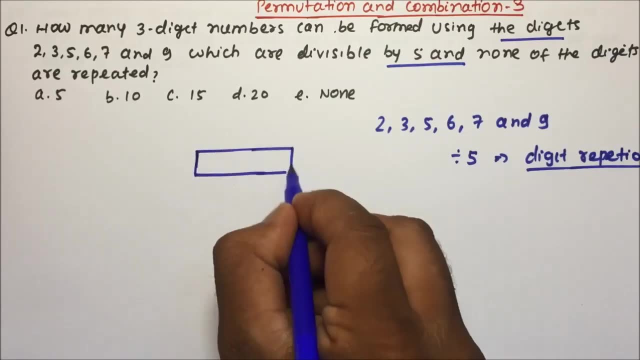 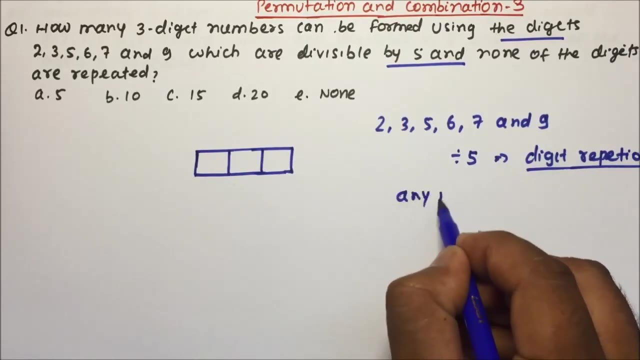 not getting repeated Digits. repetition is not there and digit repetition is not there, Right, friends? okay, Now you want 3 digit number, You want 3 digit number, and that 3 digit number should be divisible by 5.. So if any number, if any number is divisible by 5, so if any number is divisible, 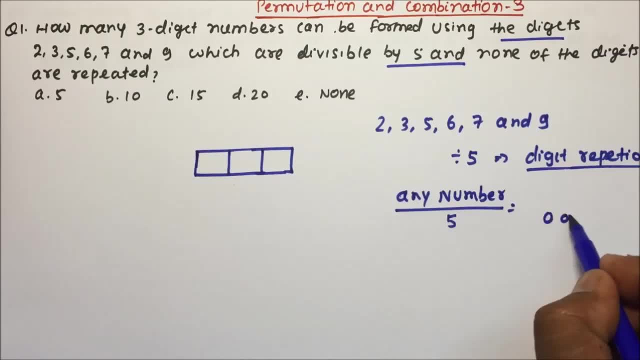 by 5, then the number should end with 0 or 5.. The number should end with 0 or 5.. But you see, we have 6 digit and there is no 0. We have 6 digit, but there is no 0. So I can say: 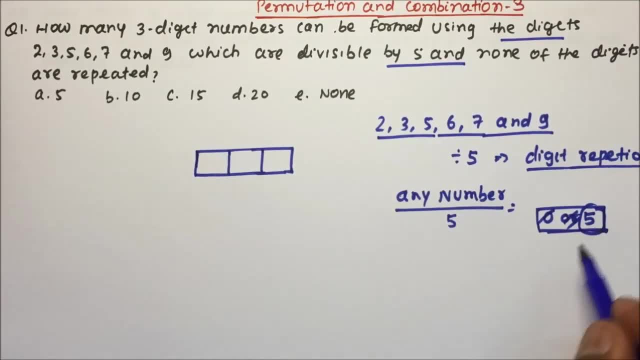 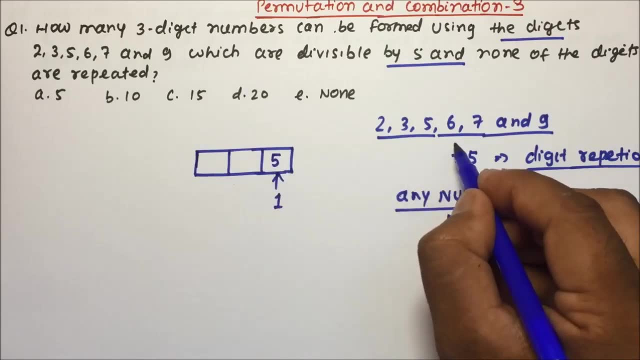 here the number should end with 5.. Here the number should end with 5.. So, friends, I can say here that I have only one choice to put the digits. here I can put only 5 here. I can put only 5 here. 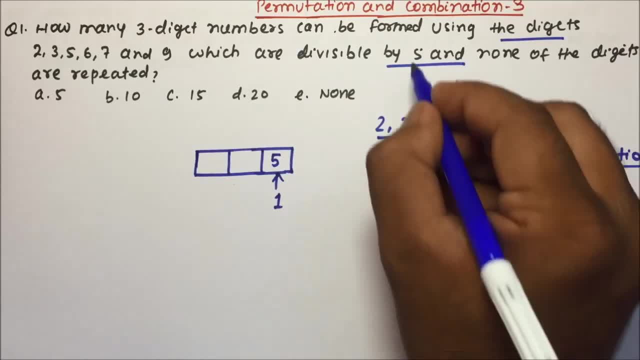 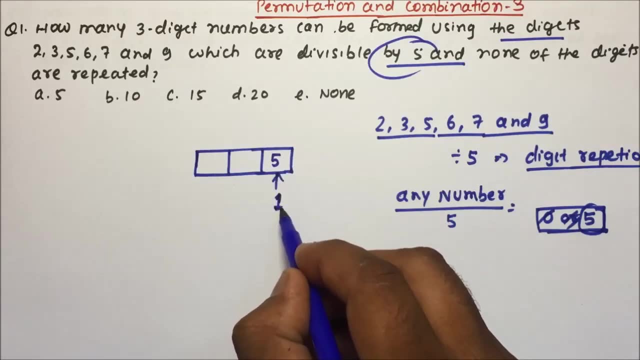 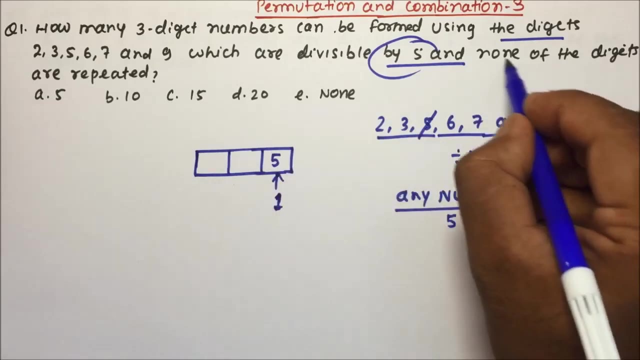 I cannot put any other number because the number has to be divisible by 5, and if a number is divisible by 5, then it should end with 5.. So I have only one choice. I have only one choice. okay, Now, 5 already we are putting here, So the same 5 should not repeat, because in the question 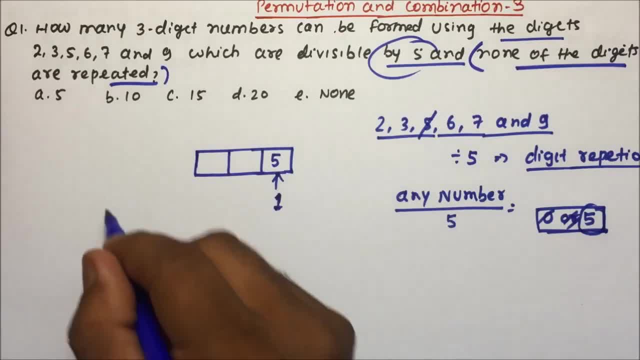 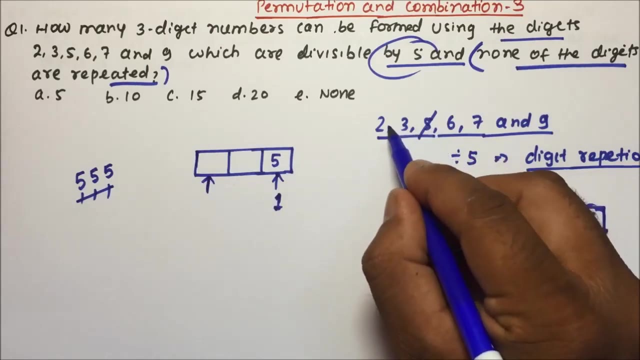 they are clearly telling: none of the digit is repeated Means we cannot have a number 555.. We cannot have a number 555 because here the numbers, digits, are repeated. okay, friends Now. so how many options we have here? So 5, we cannot put After that 1, 2,, 3,, 4, 5.. So after: 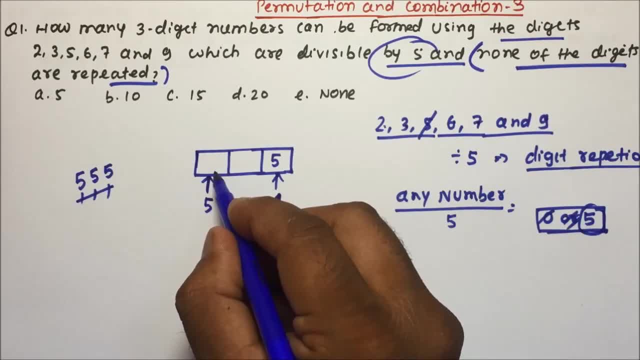 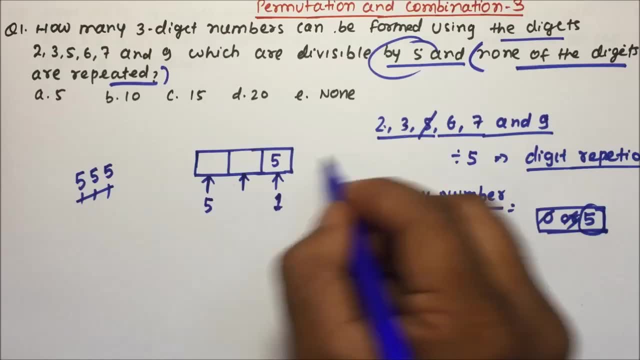 that I have 5 choice. Out of that 5 choice, I can put any digit here. I can put any digit here and then next friends, and then next how many choices will be there? So suppose you are putting 2 here, then I will be left with, then I will be left with 5.. So I can put any digit here and then next. 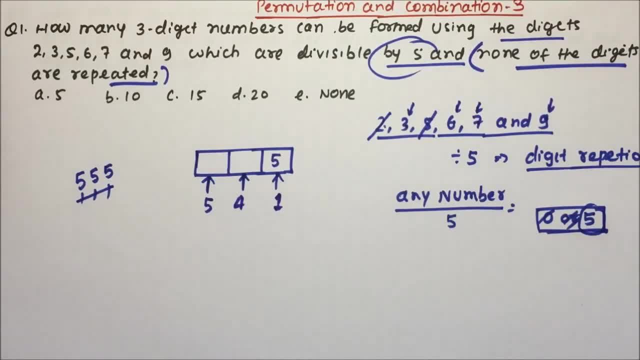 next, how many choices will be there? So suppose you are putting 2 here, then I will be left with with only 4 choice. So out of this 4 choice I can put 1 digit here. So in that case, friends, 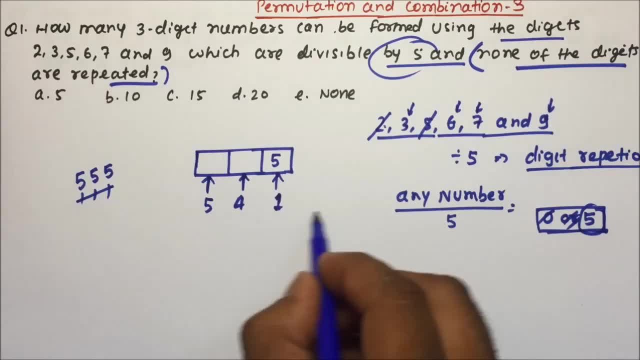 none of the digits will be repeated and we will be getting the 3 digit number which is divisible by 5.. So the total number, so the total number, friends, I can say 5 into 4 into 1. So the total number will be 20.. So there are total, 3 digit number is 20, which will 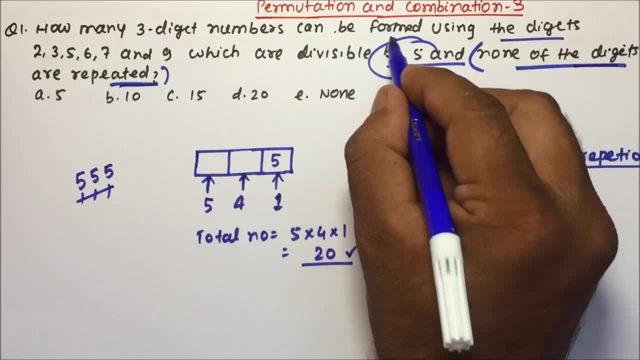 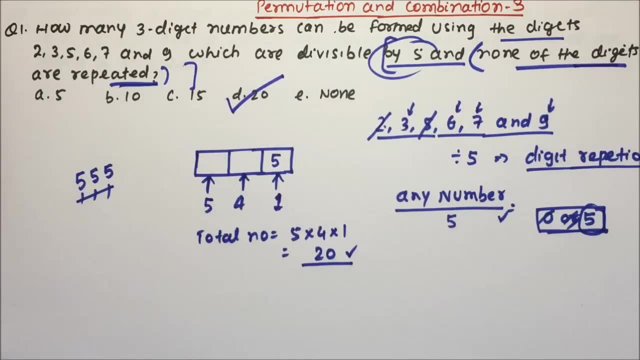 be divisible by 5 and none of the digits are repeated. So there was 2 condition was there and both the condition we have covered here. So option D will become the correct answer for question number 1.. Now moving towards the question number 2.. 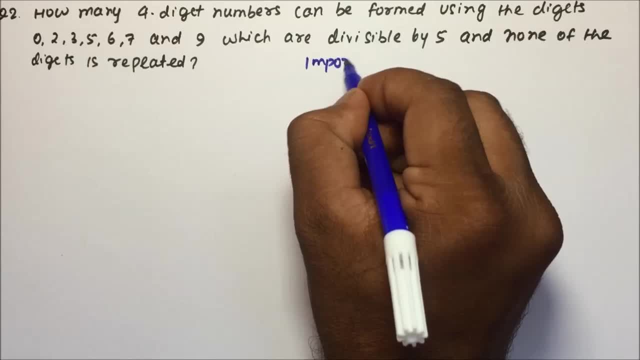 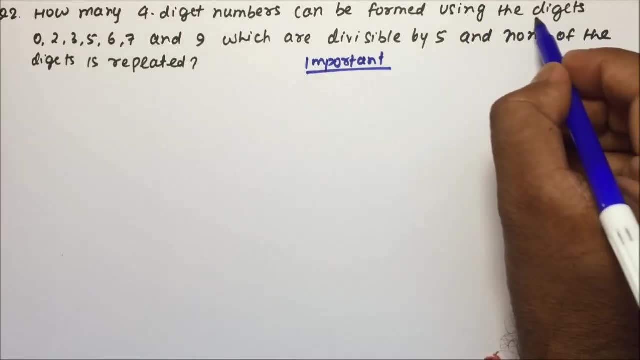 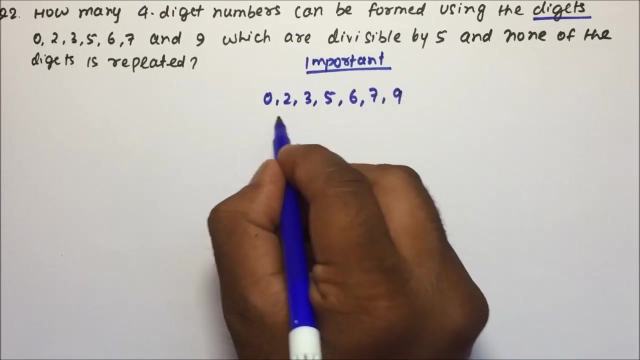 Now, friends, question number 2, question number 2 is also important and there is little twist in this question, so that you have to understand. So how many 4 digit number can be formed using the digits 0,, 2,, 3,, 5,, 6,, 7 and 9.. So, using this digit, we are going to get the total number. 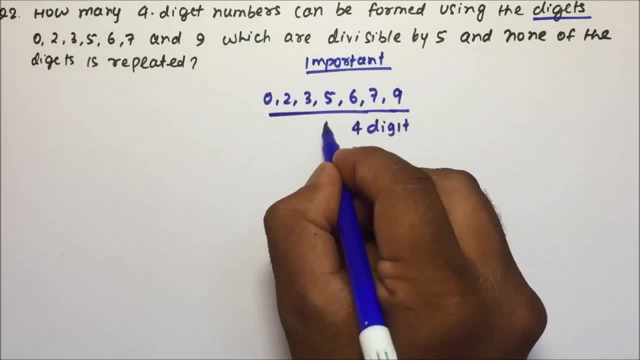 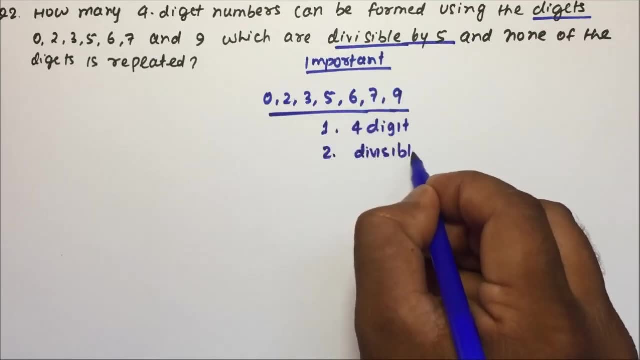 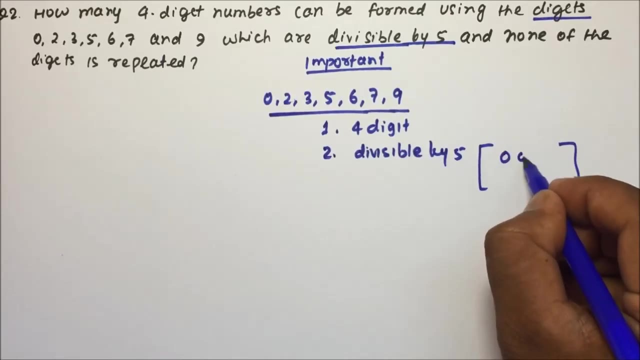 going to form a 4 digit number. So first condition is the number should be 4 digit, and the second condition is: which are divisible by 5, and the second condition is: divisible by 5, divisible by 5. okay, friends, Now we know. if any number is divisible by 5, then 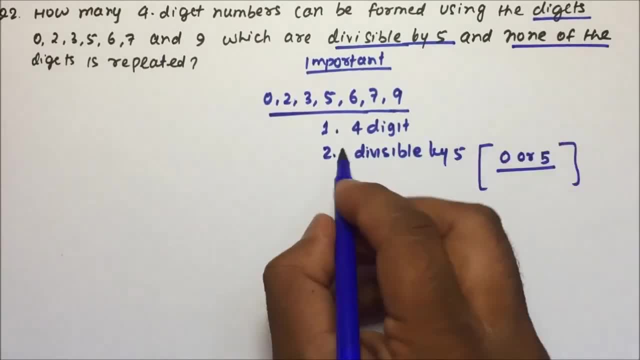 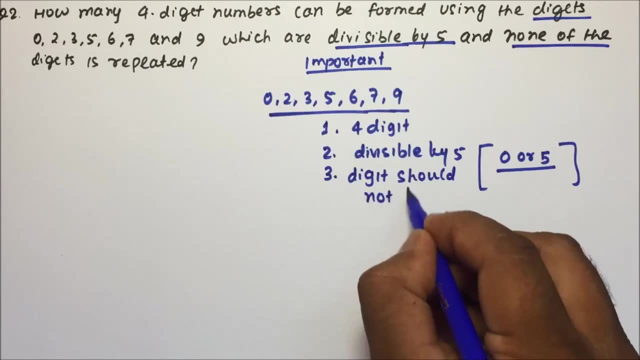 the last digit should be 0 or 5. and, friends, we have one more condition: that digit should not be repeated. digit should not be repeated, digit should not be repeated. So, keeping all the conditions, So keeping all the conditions in mind, we are going to frame a 4 digit number. So my 4 digit, 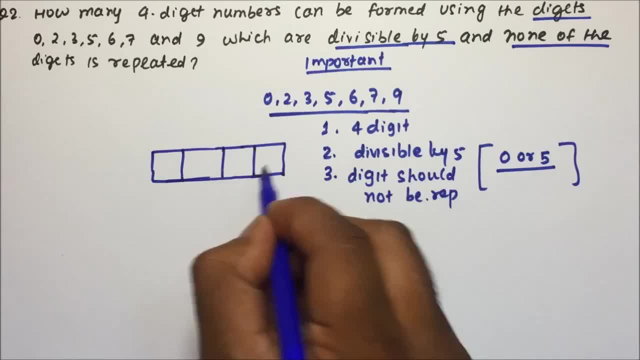 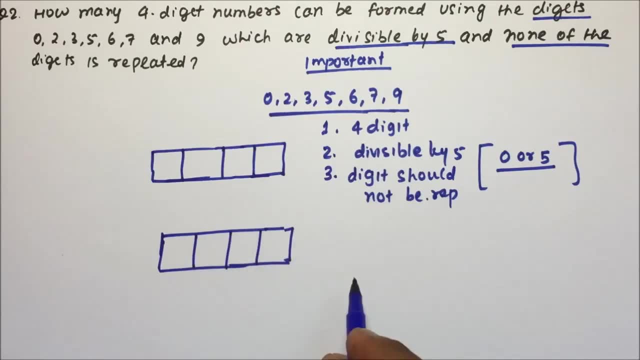 number 1,, 2,, 3 and 4.. I am making one more box. I will tell you the reason why I have made 2 box: 1,, 2,, 3 and 4.. Now, if you want the numbers to be divisible by 5, then you. 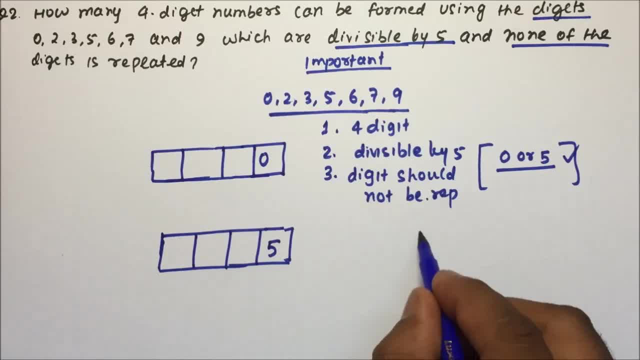 can put 0 or you can put 5.. Now, friends, why I have not taken, why I have not taken only one box, that I will tell you. See, the reason is Because, if you are putting 5 here and if you are considering only one box and you are telling, 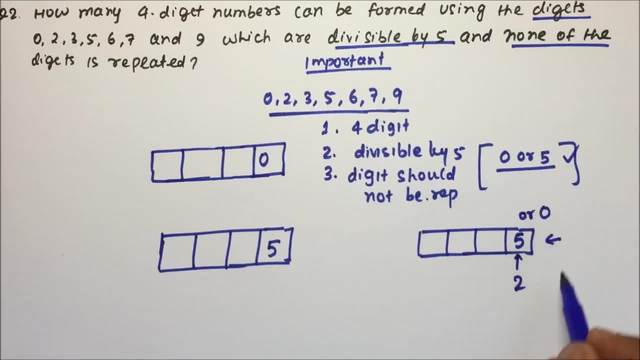 you have 2 choice, that either you can put 5 or you can put 0. So if you are putting 5 here and if you are putting 0 here, then this number will become. then this number will be no more a 4 digit number, because a 4 digit number cannot start with 0. So that is the. 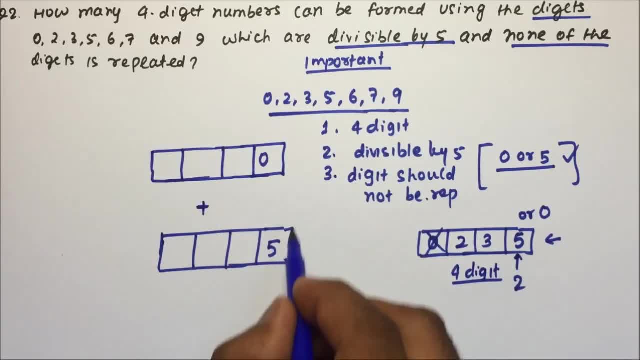 only reason. I have taken 1 with 0 and I have taken 1 ending with 5, so that we will be getting the numbers which is divisible by 5. And then later on we will add it Now, friends. so with 0, I have only 1 choice. I can put 0.. 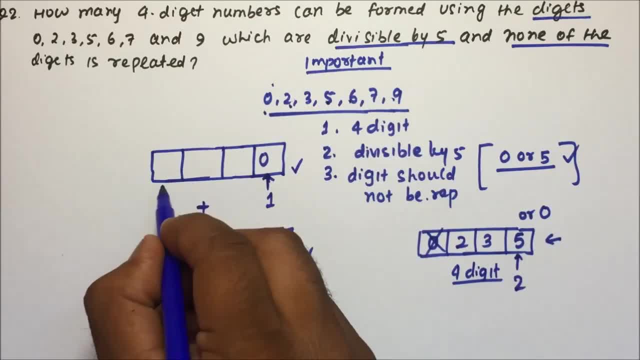 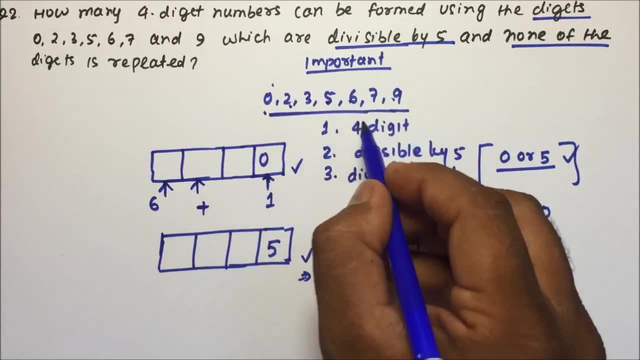 So once you will put 0, then after that how many options will be there? 3 plus 3. 6. So I can use any of the 6 option here Then. so suppose if you are putting 2 here, then how many options you will be having? 1,. 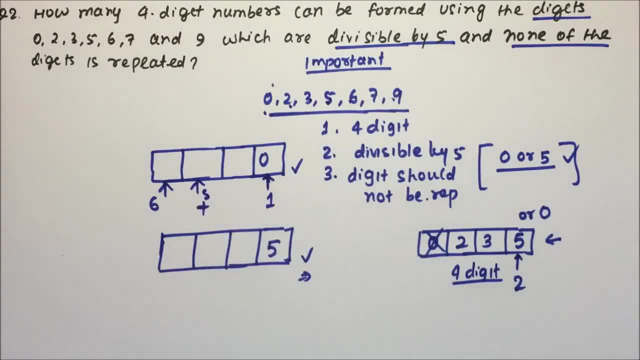 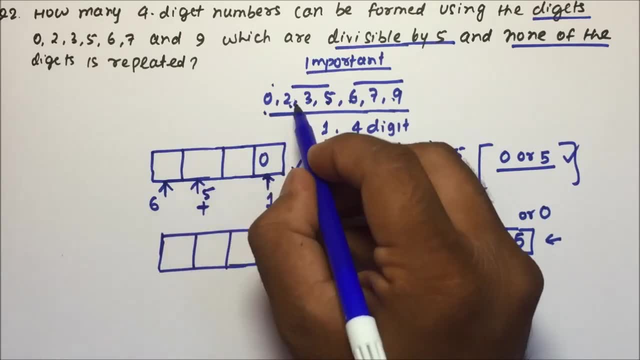 2,, 3,, 4, 5.. Then you will be having 5 options. See, friends, try to understand. you will put 0 here, then you will have 3 plus 3, 6 option, so any 6 choice you can put it here. So suppose you are putting. 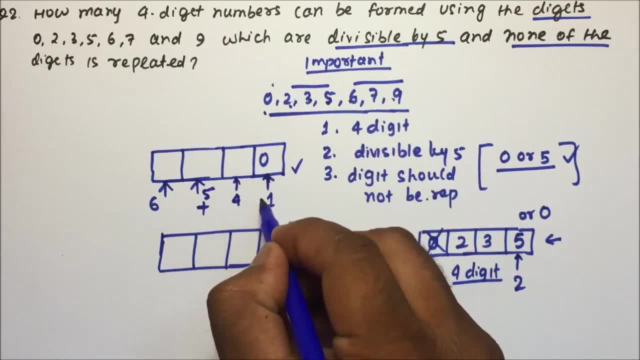 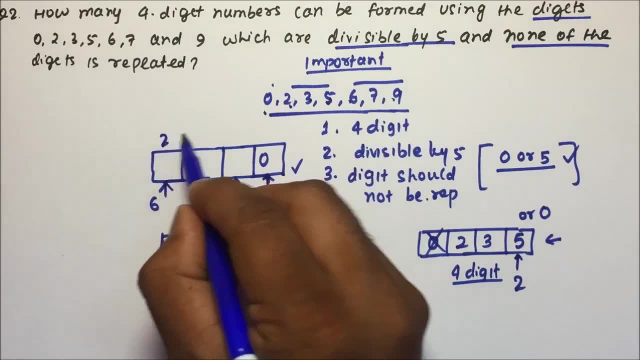 put 2 here. so after that, how many choice? 5, after that, how many choice will be having? 4? because choice will be reducing. for you, right, friends? because digit does not have to repeat. so if you are putting 2 here, you cannot put 2 here, you will have to use whatever. 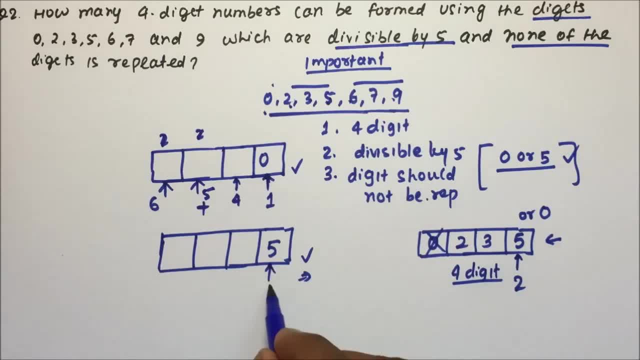 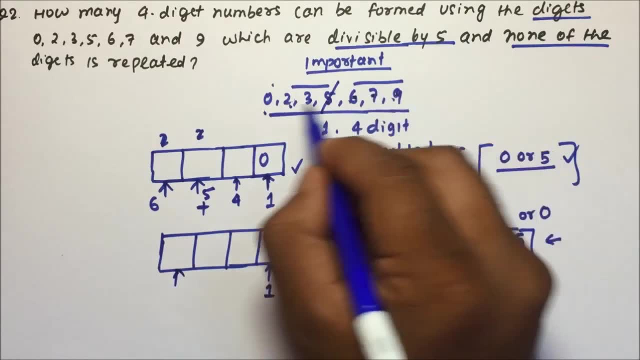 the digit remaining. Now, friends, if the number is ending with 5, then there is only one choice. you can put 5 here now. after that, how many choice will have? 1,, 2,, 3,, 4,, 5, 6? you have 6 choice, but 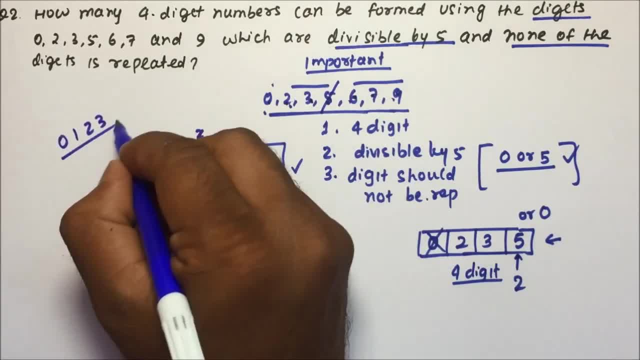 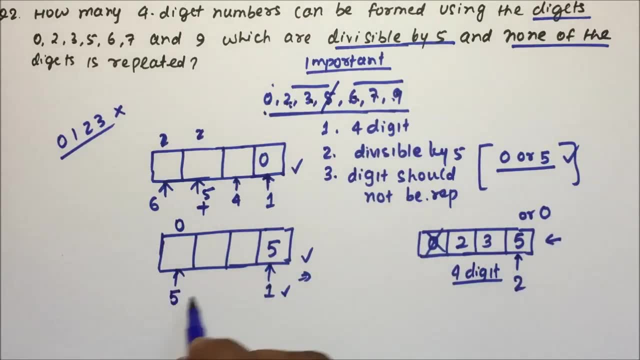 you cannot put 0 here, because if a number will start with 0, it can never be a 4 digit number, so 0 also you cannot put here. so 1,, 2,, 3,, 4, 5, so you will have 5 choice. then 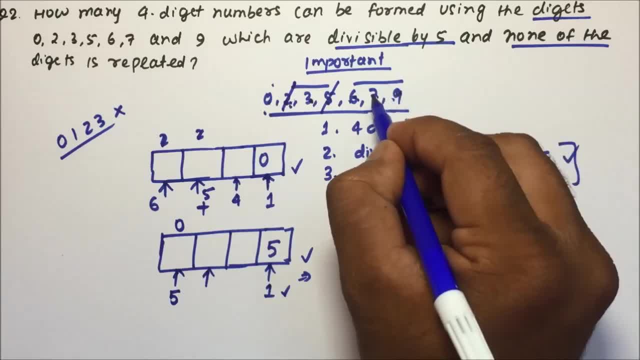 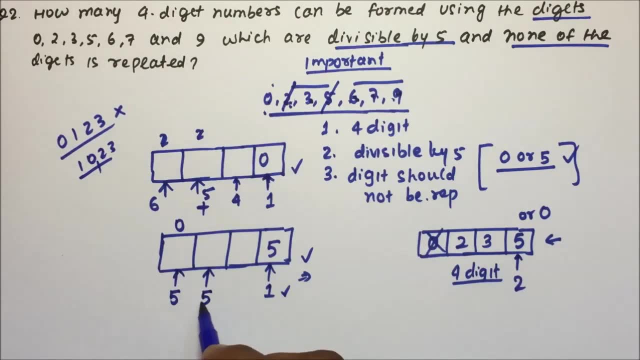 suppose you have put 2 here, then how many choices will be left for you? 1,, 2, 3, 4, 5. but 0 I can put at the second place, no problem. so again you will have 5 choice, and then friends.